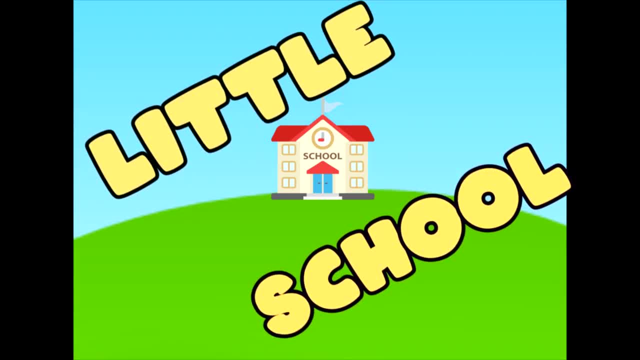 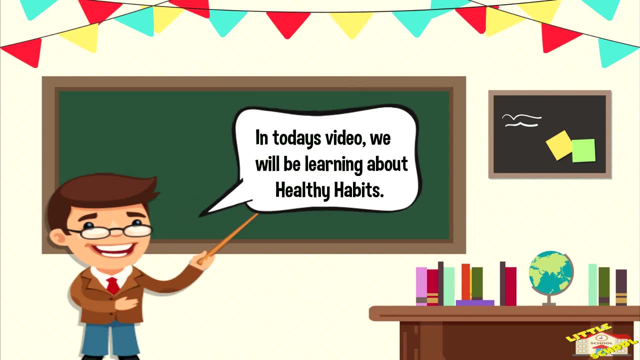 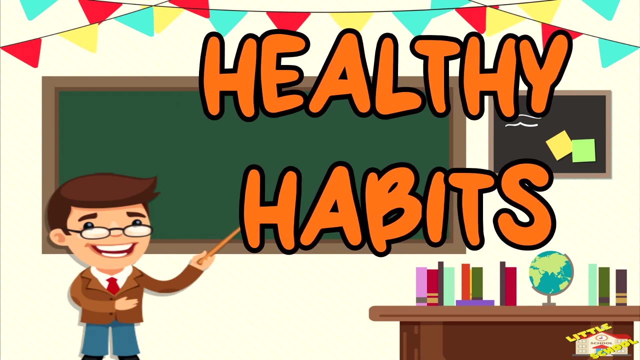 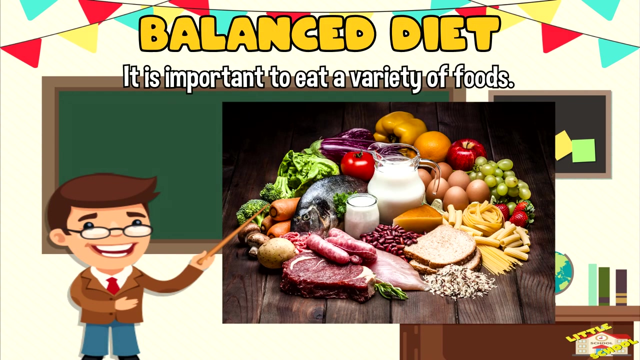 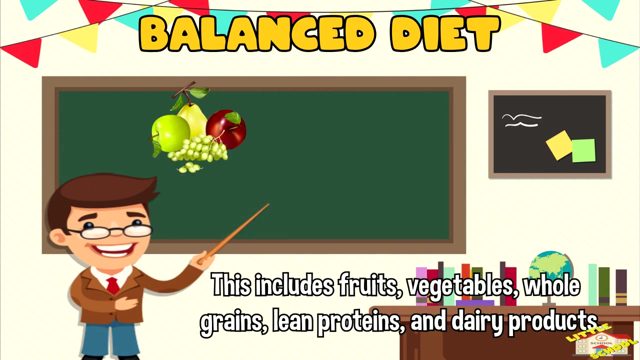 Hey kids, In today's video, we'll be learning about healthy habits. Are you ready? Let's begin A balanced diet. It is important to eat a variety of foods. This includes fruits, vegetables, whole grains, lean proteins and dairy products. 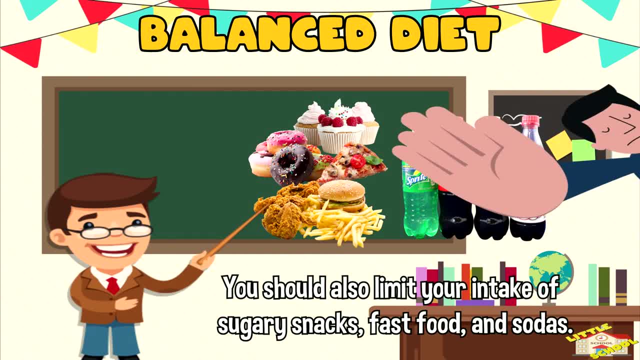 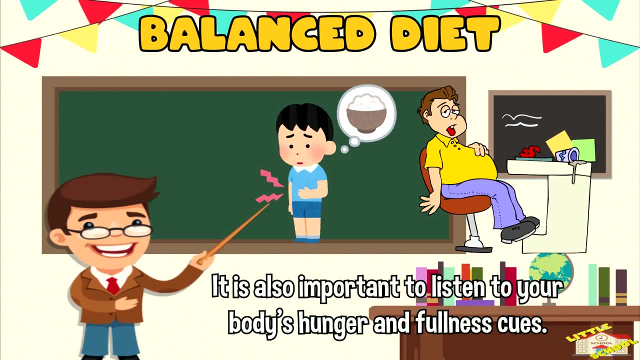 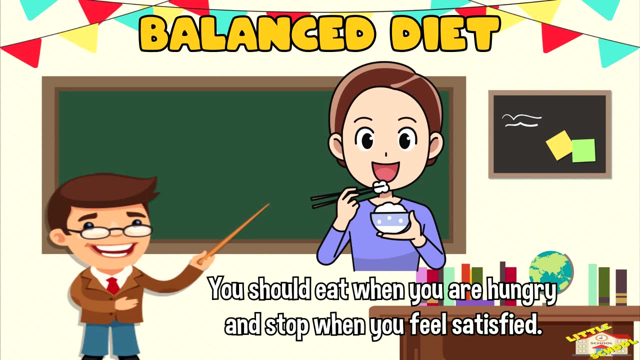 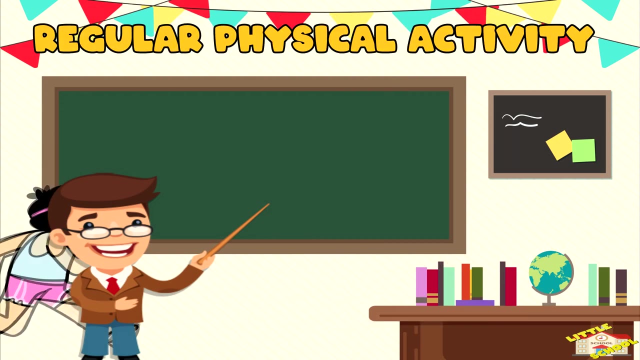 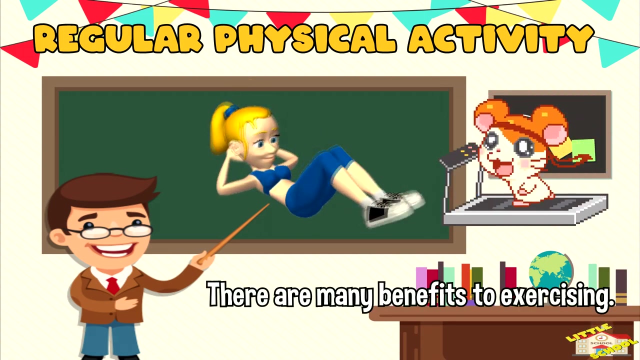 You should also limit your intake of sugary snacks, fast food and sodas. It is also important to listen to your body's hunger and fullness cues. You should eat when you are hungry and stop when you feel satisfied. Regular physical activity. There are many benefits to exercising. These benefits are: 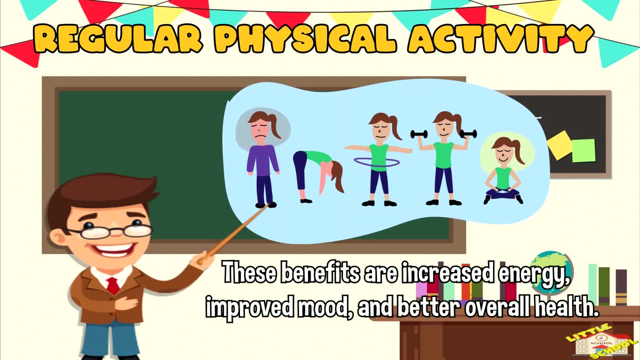 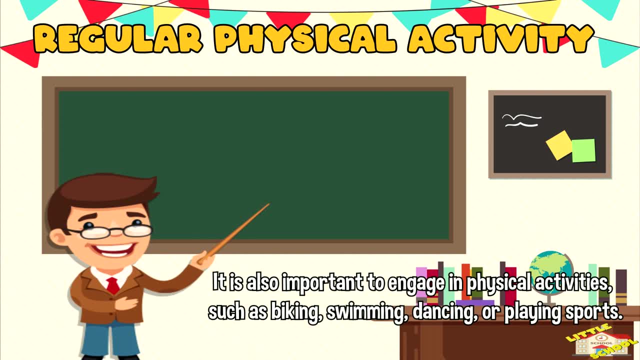 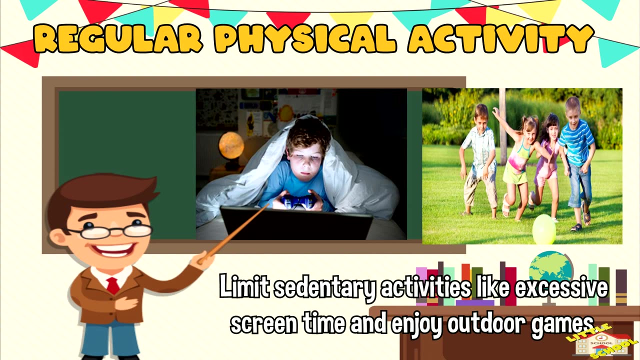 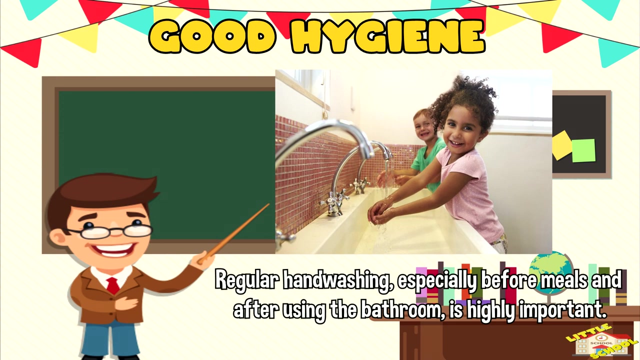 increased energy, improved mood and better overall health. It is also important to engage in physical activities such as biking, swimming, dancing or playing sports, Limit sedentary activities like excessive screen time and enjoy outdoor games. Good hygiene- Regular hand washing, especially before meals and after using the bathroom, is highly important. 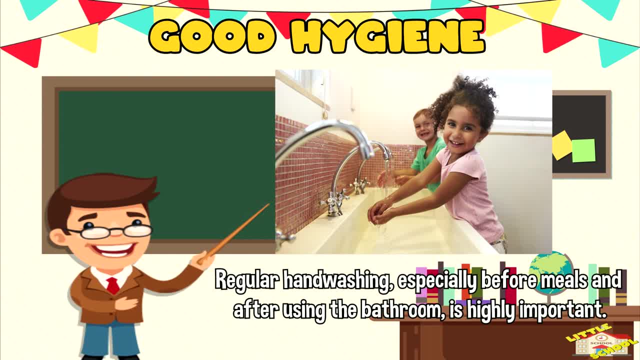 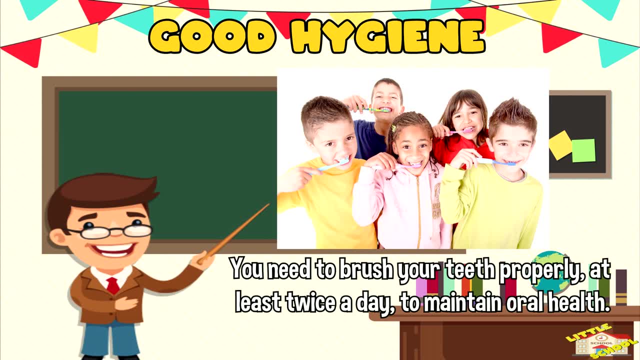 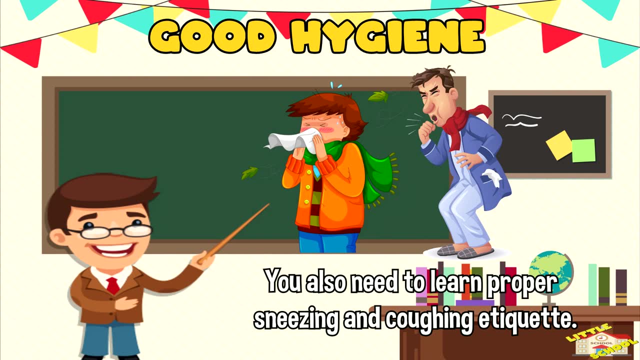 You need to brush your teeth properly at least twice a day to maintain oral health. You also need to learn proper sneezing and cuffing. You also need to learn proper sneezing and cuffing etiquette, like covering your mouth and nose with a tissue or elbow to prevent. 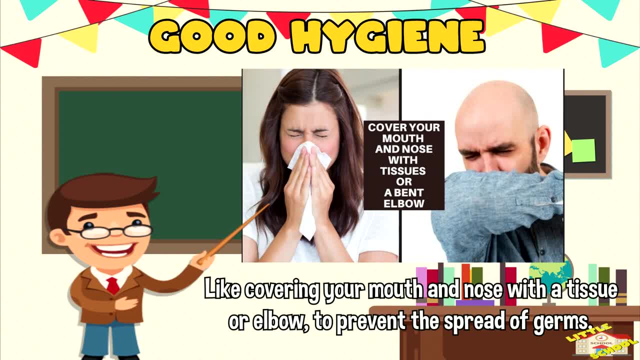 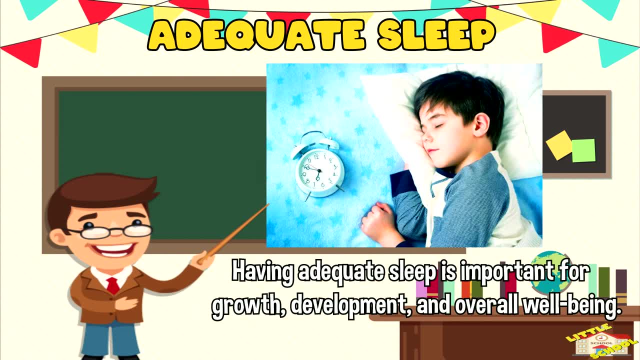 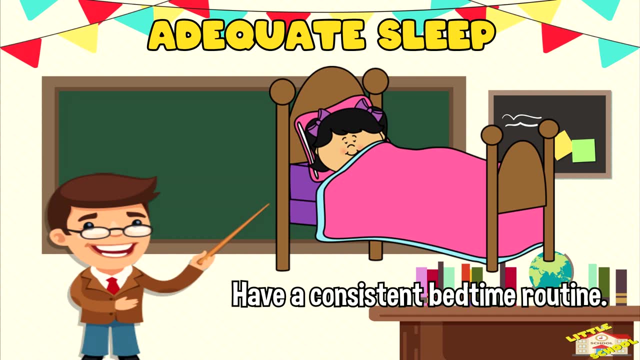 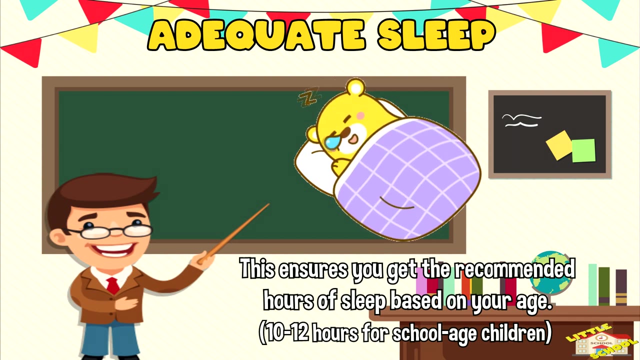 the spread of germs. adequate sleep- having adequate sleep- is important for growth, development and overall well-being. have a consistent bedtime routine. this ensures you get the recommended hours of sleep based on your age. that is 10 to 12 hours for school-aged children. create a sleep.